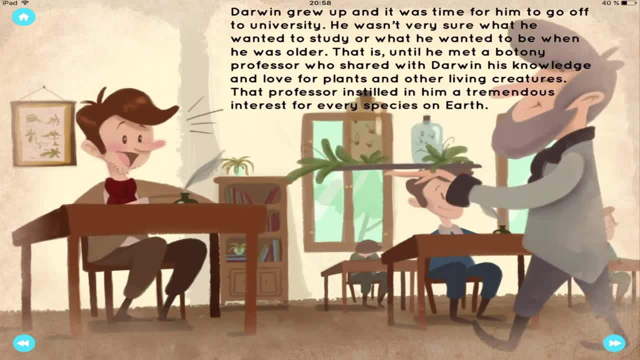 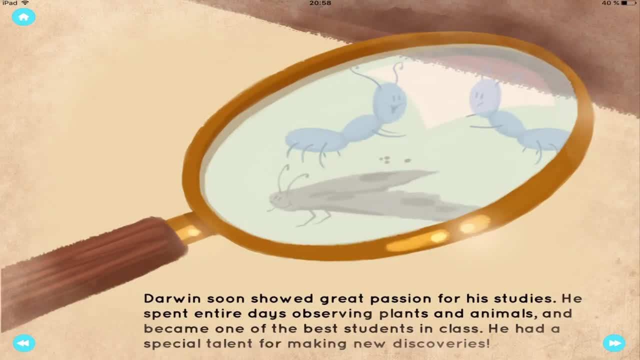 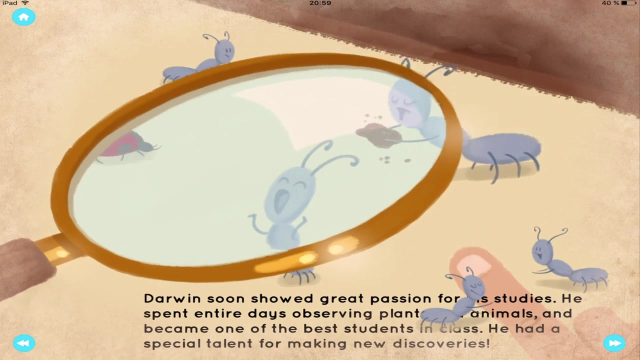 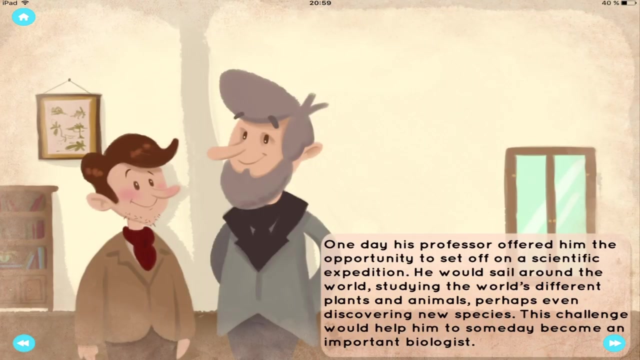 Aha Darwin soon showed great passion for his studies. He spent entire days observing plants and animals and became one of the best students in class. He had a special talent for making new discoveries. One day, his professor offered him the opportunity to set off on a scientific 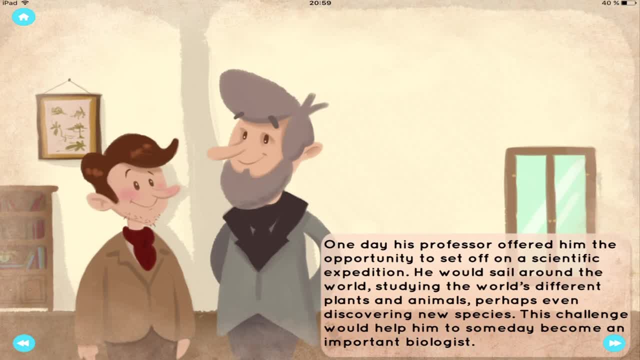 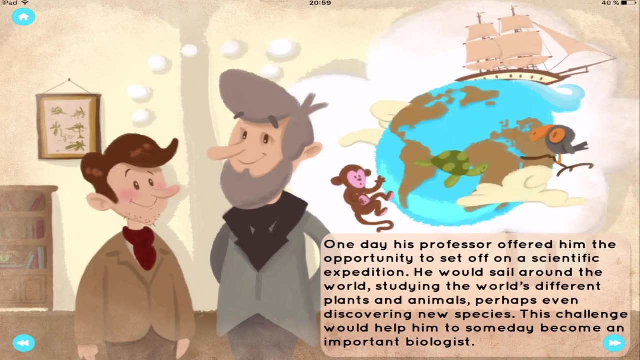 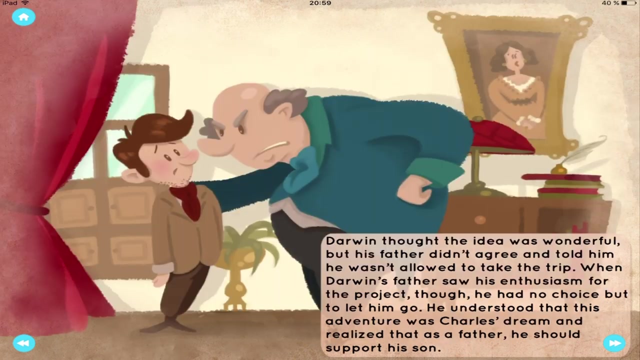 expedition. He would sail around the world studying the world's different plants and animals, perhaps even discovering new species. This challenge would help him to someday become an important biologist. Darwin thought the idea was wonderful, but his father didn't agree and told him he wasn't allowed to take the trip. When Darwin's father saw his enthusiasm for 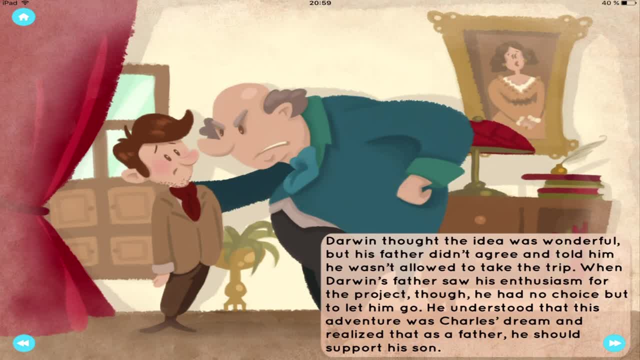 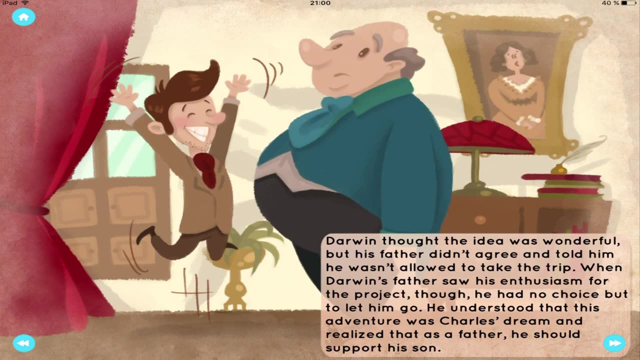 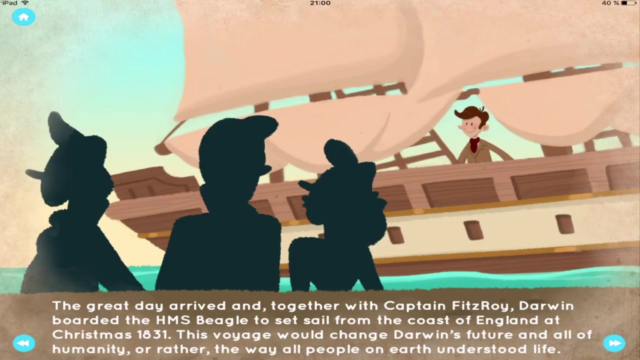 the project, though he had no choice but to let him go. He understood that this adventure was Charles's dream and realized that, as a father, he should support his son. The great day arrived and, together with Captain Fitzroy, Darwin, boarded the HMS Beagle to set sail from the coast of England at Christmas 1831. This voyage, 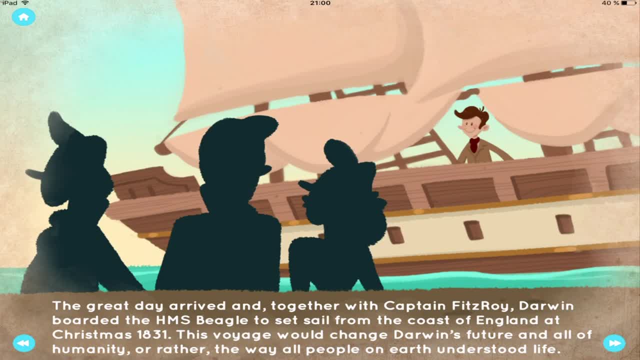 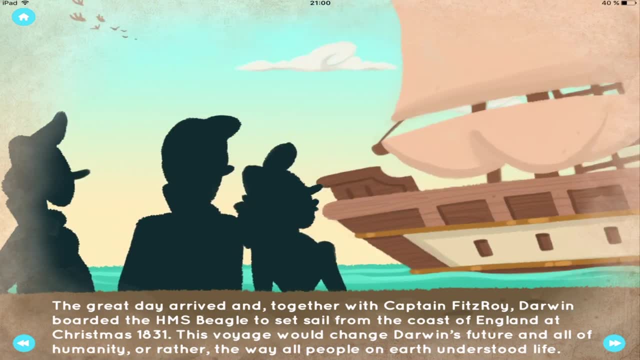 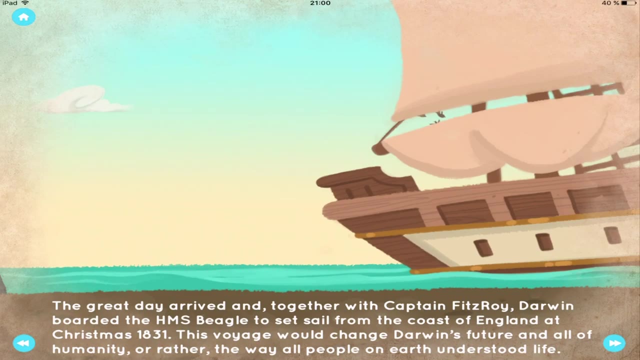 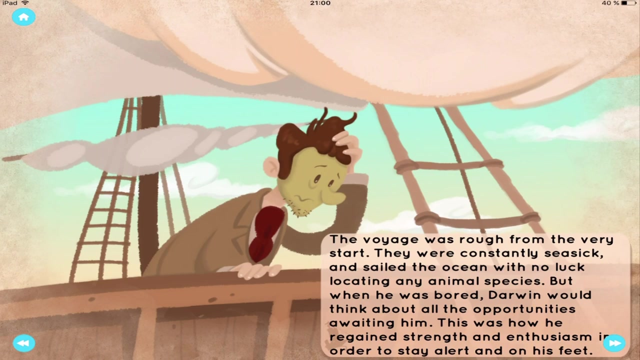 would change Darwin's future and all of humanity, or rather the way all people on earth understood life. The voyage was rough from the very start. They were constantly seasick and sailed the ocean with no luck locating any animal species. But when he was bored, 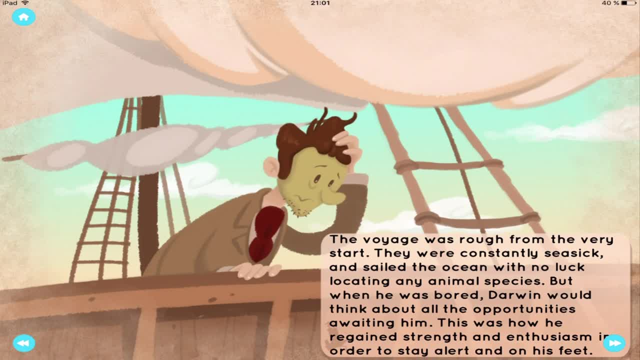 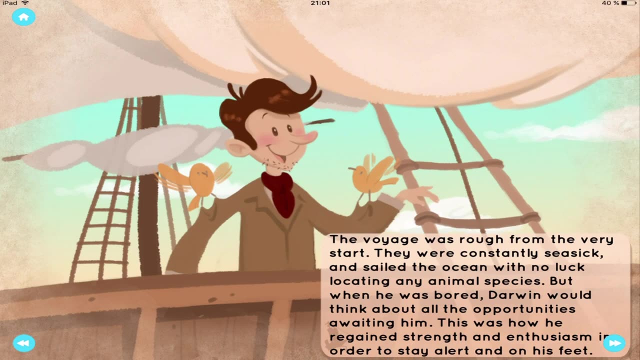 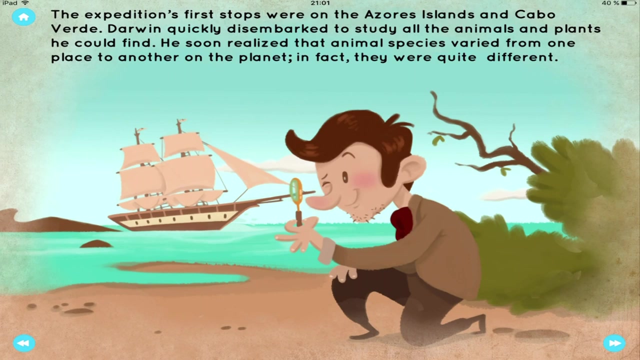 Darwin would think about all the opportunities awaiting him. This was how he regained strength and enthusiasm in order to stay alert and understand the world. The expedition's first stops were on the Osiris Islands and Cabo Verde. Darwin quickly disembarked to study all the animals and plants he could find. He soon 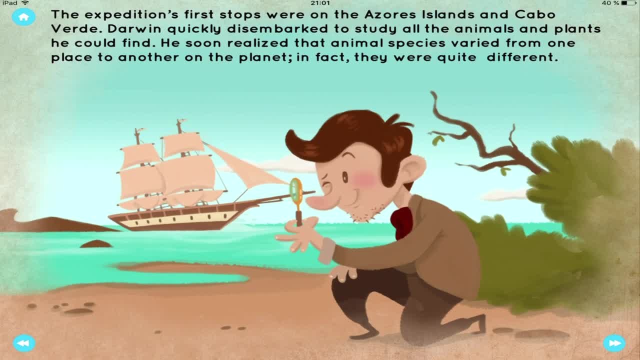 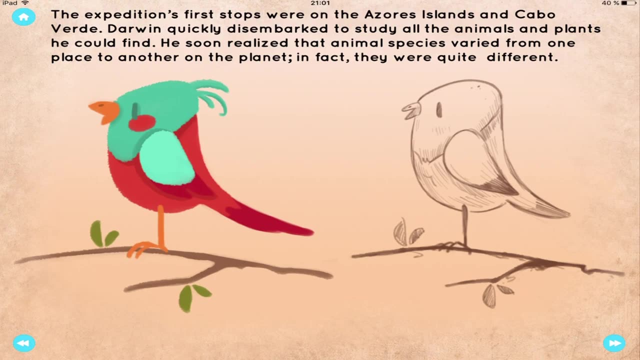 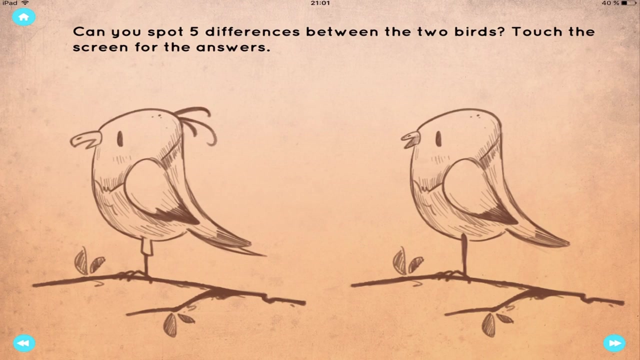 realized that animal species varied from one place to another on the planet. In fact, he had no idea what he was talking about. In fact, they were quite different. Can you spot five differences between the two birds? Touch the screen for the answers. 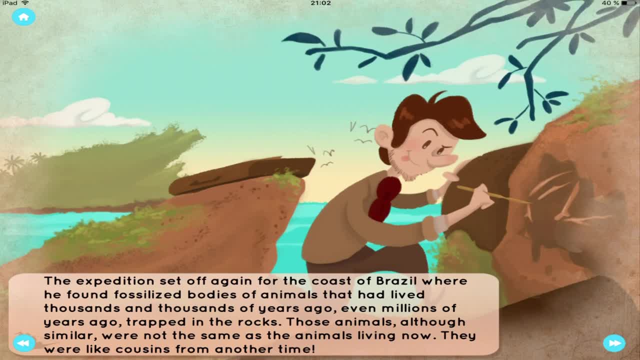 The expedition set off again for the coast of Brazil, where he found fossilized bodies of animals that had lived thousands and thousands of years ago, Even millions of years ago, trapped in the rocks. Those animals, although similar, were not the same as the animals living now. They were like cousins from another. 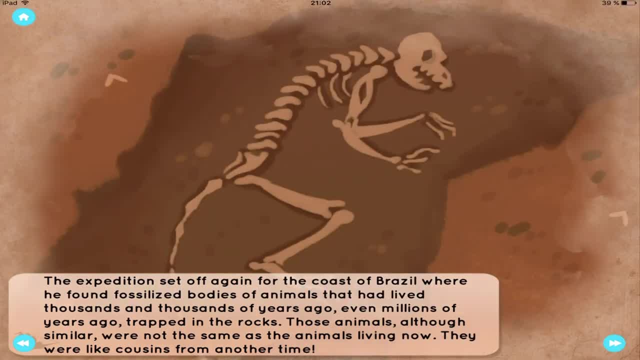 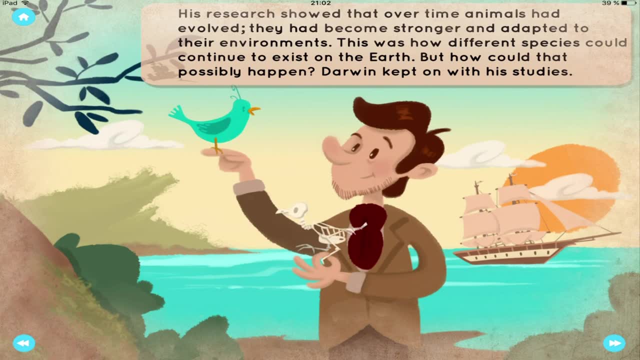 time. His research showed that over time, animals had evolved. They had become stronger and adapted to their environments. This was how different species could continue to exist on the Earth. But how could that possibly happen? Darwin kept on with his studies. 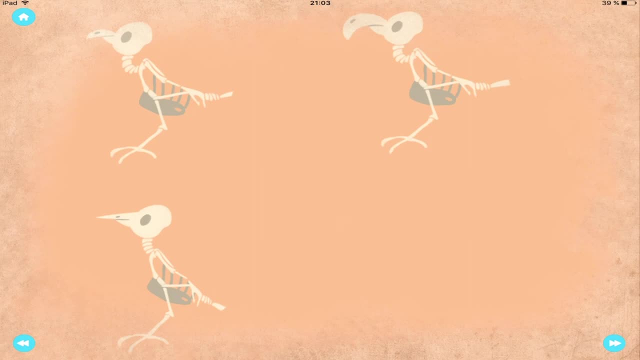 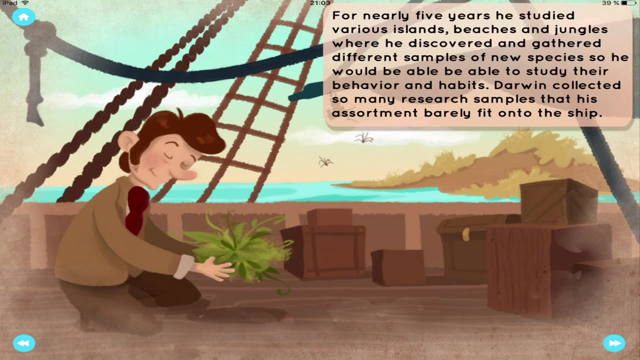 For nearly five years he studied various islands, beaches and jungles where he discovered and gathered different samples of new species so he would be able to study their behavior and habits. Darwin collected so many research samples that his assortment barely fit onto the ship. 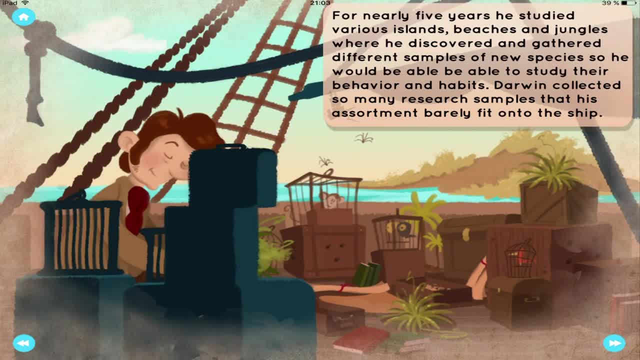 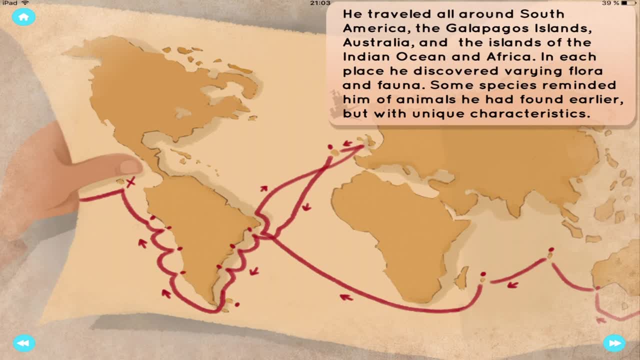 He traveled all around South America, the Galapagos Islands, Australia and the islands of the Indian Ocean in Africa. In each place he discovered varying flora and fauna. Some species reminded him of animals he had found earlier, but with unique characteristics. 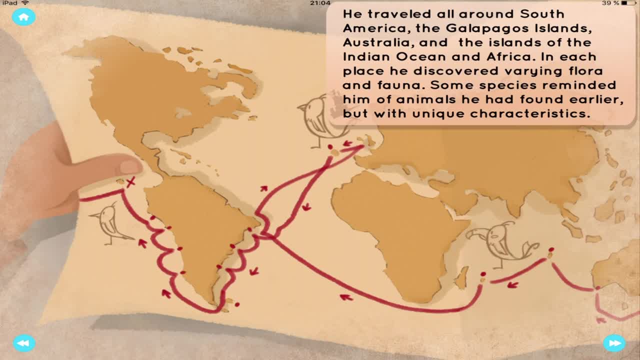 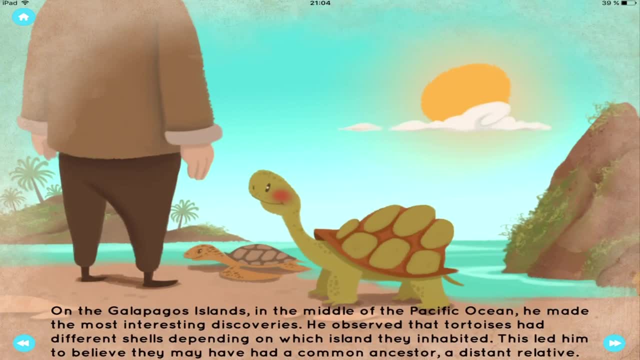 On the Galapagos Islands in the middle of the Pacific Ocean, he made the most interesting discoveries. He observed that tortoises had different shells depending on which islands they inhabited. This led him to believe they may have had a common ancestor, a distant relative. 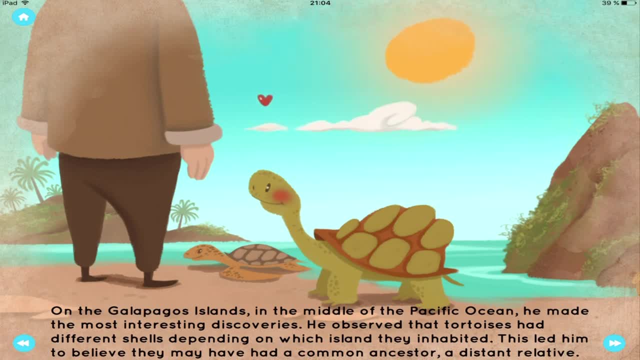 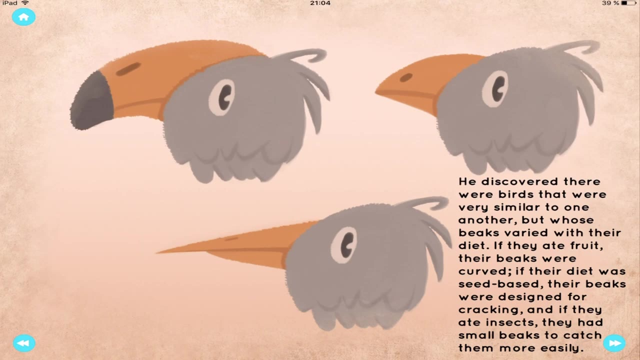 Hmm, I don't know. He discovered there were birds that were very similar to one another but whose beaks varied with their diet. If they ate fruit, their beaks were curved. If their diet was seed-based, their beaks were designed for cracking. 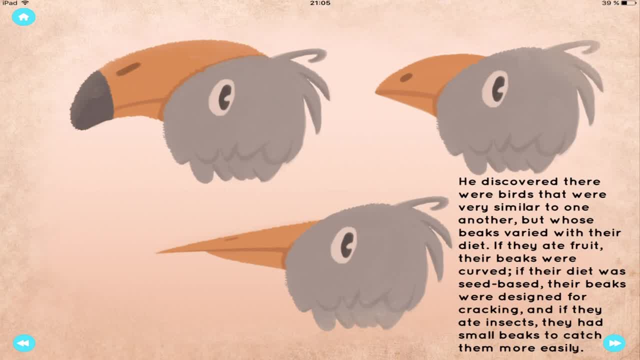 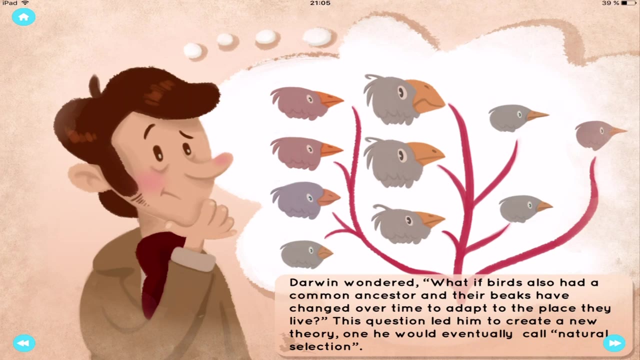 And if they ate insects, they had small beaks to catch them more easily. Darwin wondered what if birds also had a common ancestor and their beaks have changed over time to adapt to the place they live? This question led him to create a new theory, one he would eventually call natural selection. 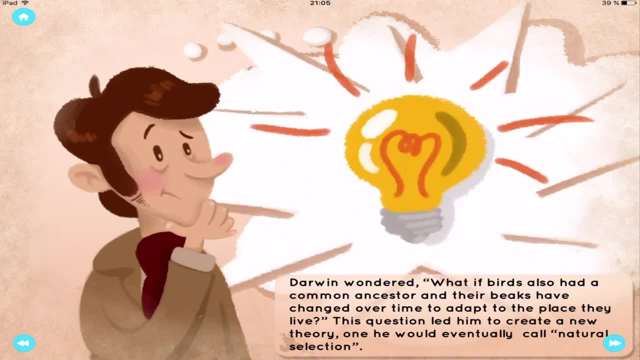 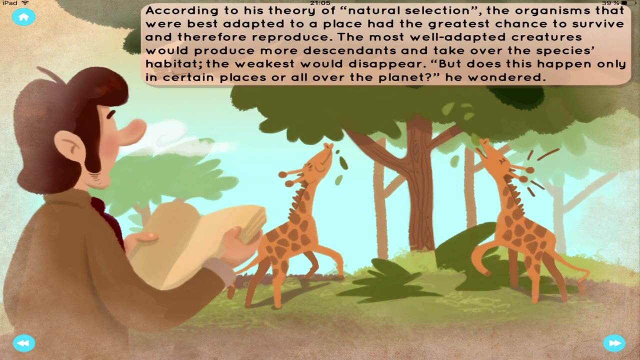 The theory that the beaks have changed over time is called natural selection, Aha. According to his theory of natural selection, the organisms that were best adapted to a place had the greatest chance to survive and therefore reproduce. The most well-adapted creatures would produce more descendants and take over the species'. 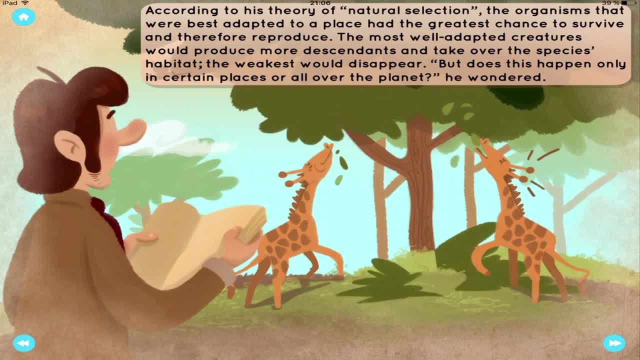 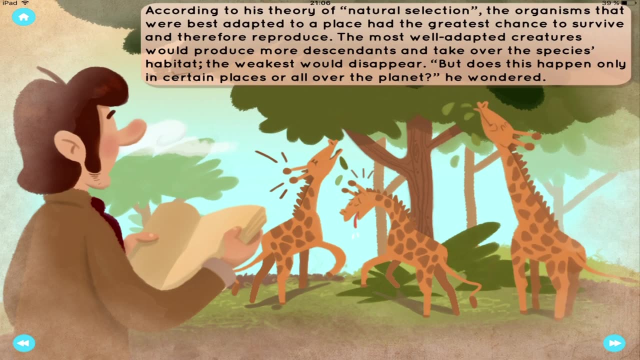 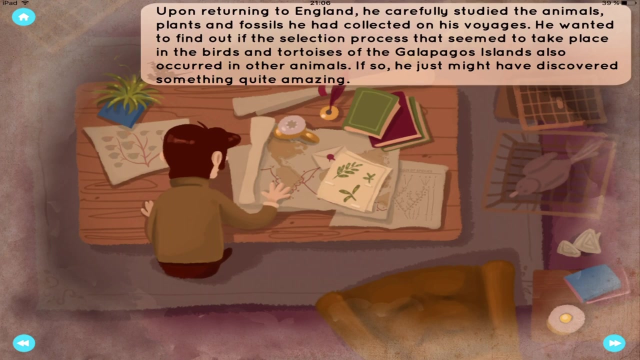 habitat, The weakest would disappear. But does this happen only in certain places or all over the planet, he wondered. Oh, Upon returning to England, he carefully studied the animals, plants and fossils he had collected on his voyages. He wanted to find out if the selection process that seemed to take place in the birds and 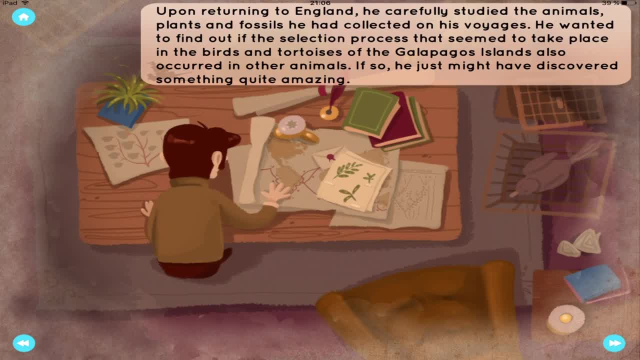 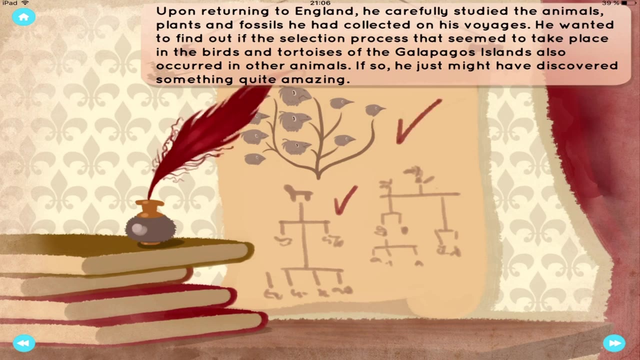 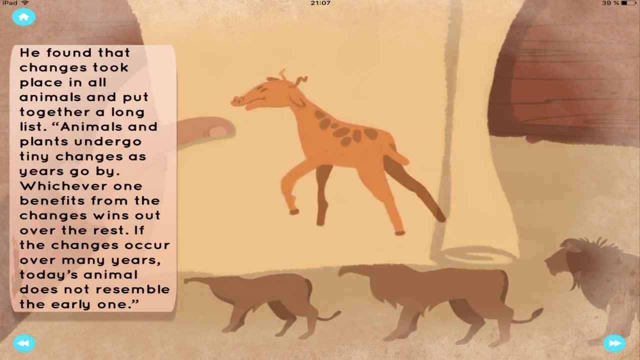 tortoises of the Galapagos Islands also occurred in other animals? If so, he just might have discovered something quite amazing. He found that changes took place in all animals. He found that changes took place in all animals. If so, he just might have discovered something quite amazing. 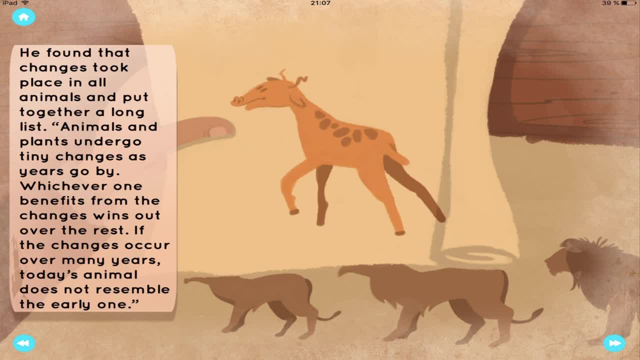 He found that changes took place in all animals. Today, animals and plants undergo tiny changes as years go by. Whichever one benefits from the changes wins out over the rest. If the changes occur over many years, today's animal does not resemble the early one. 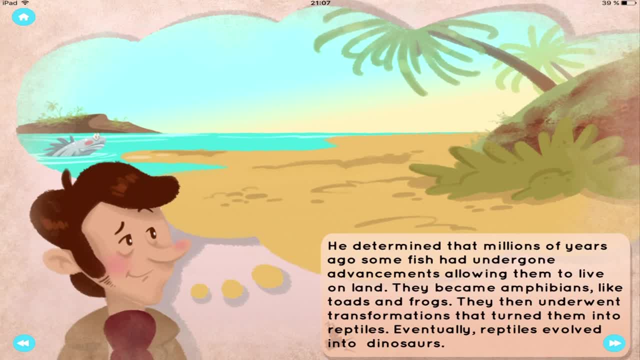 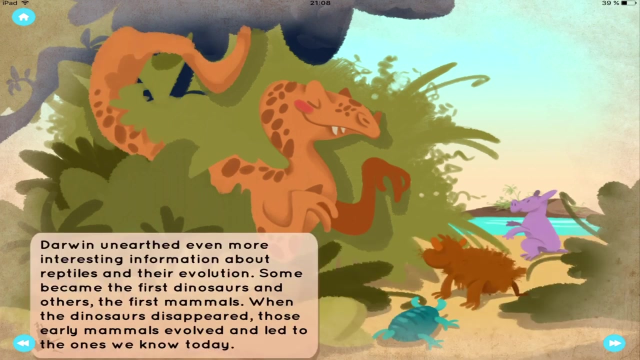 He determined that millions of years ago, some fish had undergone advancements allowing them to live on land. They became amphibians like toads and frogs. They then underwent transformations that turned them into reptiles. Eventually, reptiles evolved into dinosaurs. Darwin unearthed even more interesting information about reptiles and their evolution. 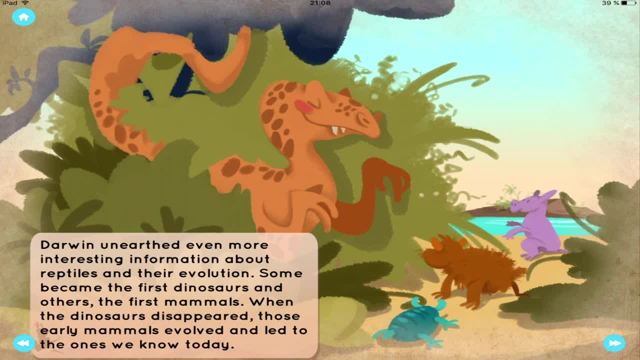 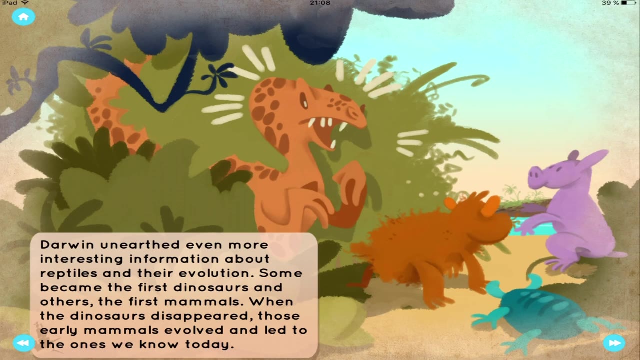 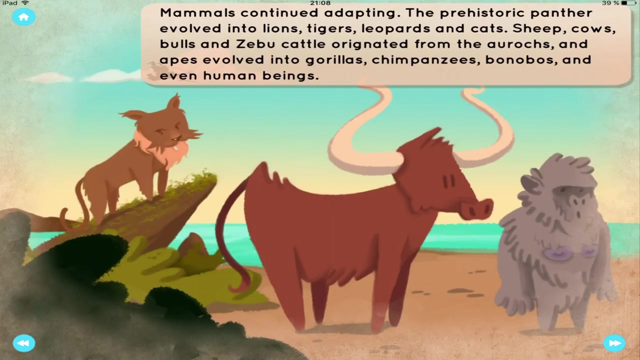 Some became the first dinosaurs and others the first mammals. When the dinosaurs disappeared, those early mammals evolved and led to the ones we know today. Mammals continued adapting. The prehistoric panther evolved into lions, tigers, leopards and cats.